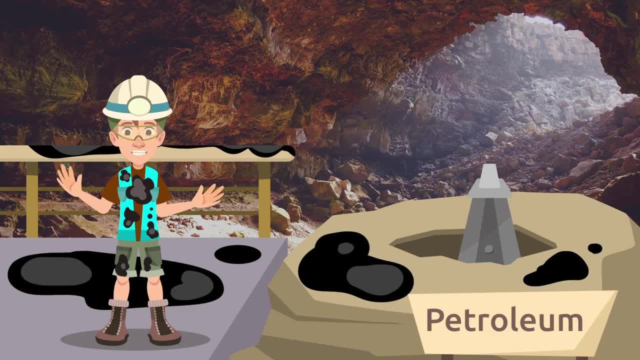 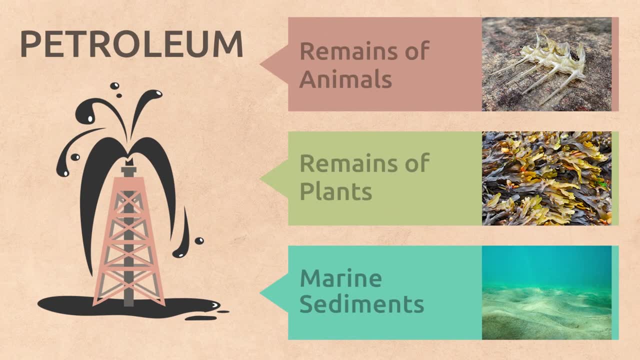 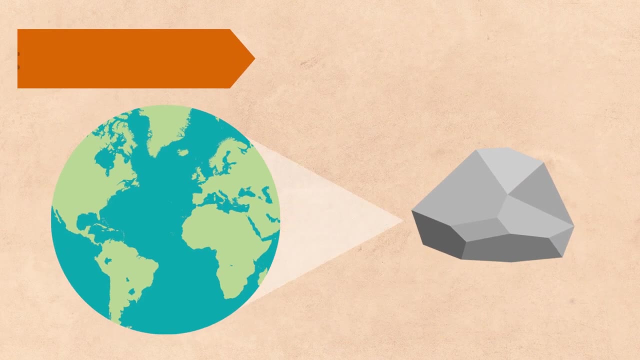 Did you know that petroleum, even though it's liquid, is a rock too? Petroleum is formed from the remains of living things like animals and plants and from sediment deposits found in marine beds. Rocks are extracted from the surface of the Earth in quarries or they are mined underground. 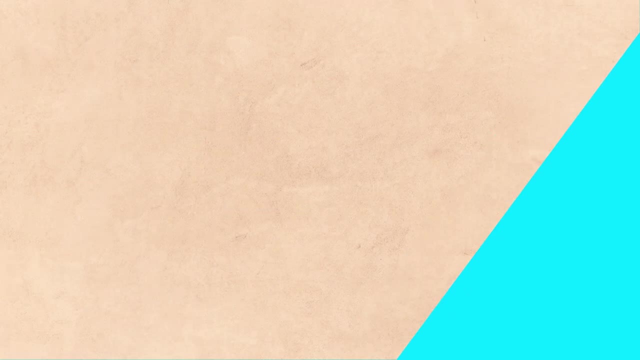 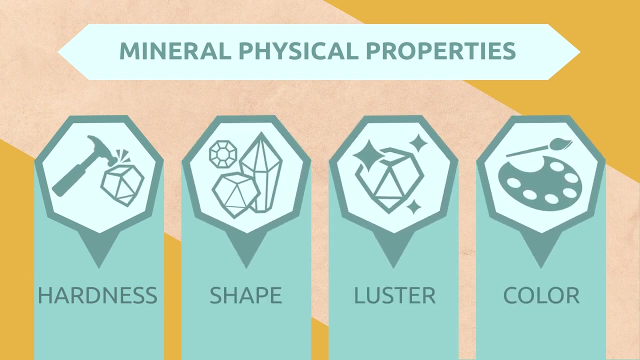 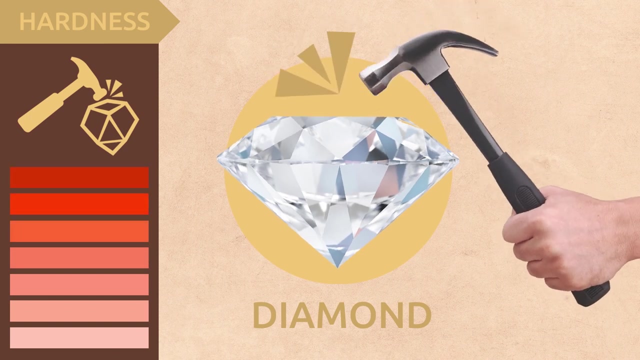 Minerals are very different from each other and have important physical properties: Hardness, shape, luster and color. Come with me, I'll show you some minerals. This one here is a diamond, the hardest mineral that exists. This one is talc, the softest mineral. 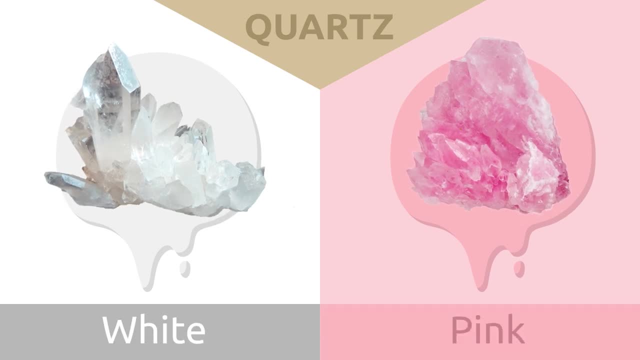 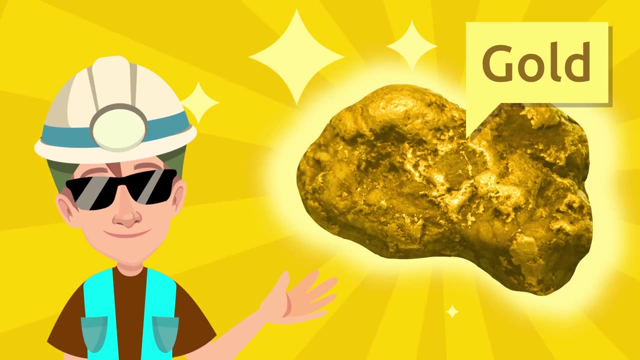 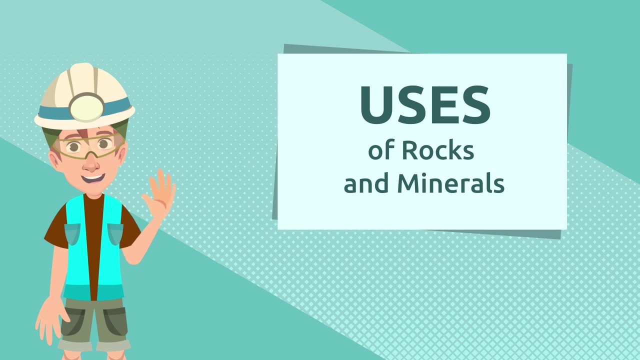 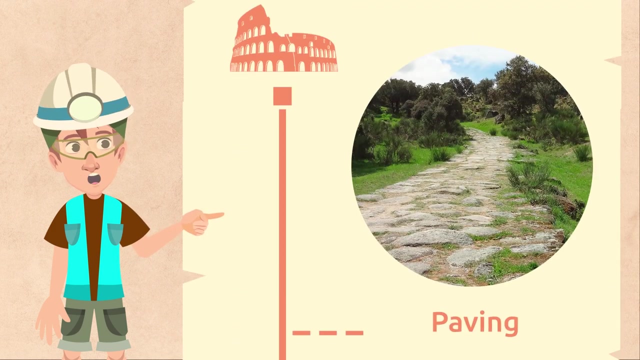 This is a quartz. It can be white or pink, And this is gold, a very shiny material. Since prehistoric times, people have used rocks and minerals for a number of things like making utensils, building their houses, paving or even making beautiful jewelry. 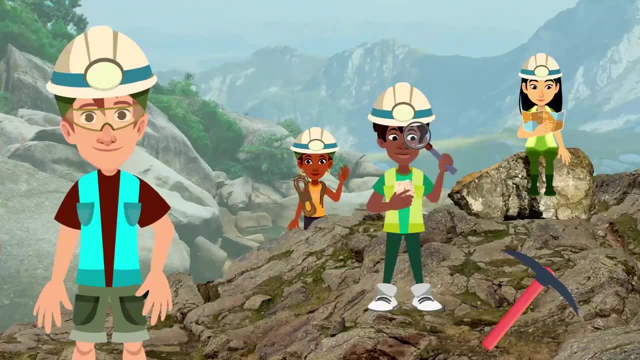 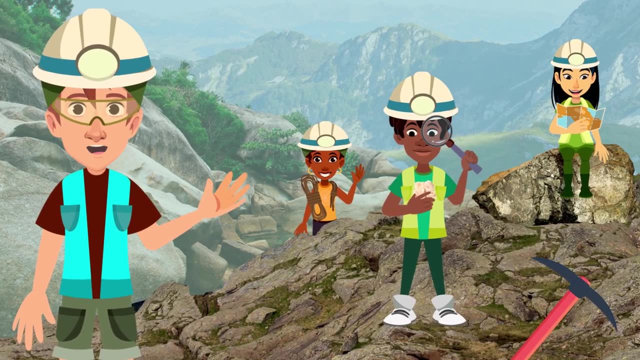 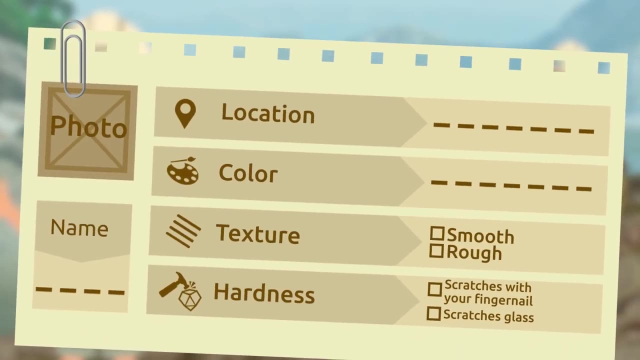 Would you like to try doing this activity? Work with your classmates and put together a rocks and minerals exposition using everything we found on our field trip. You can pick them from different places and study them in class. Tag each rock and each mineral with a label and fill it out yourselves: Name, Photo, Location. 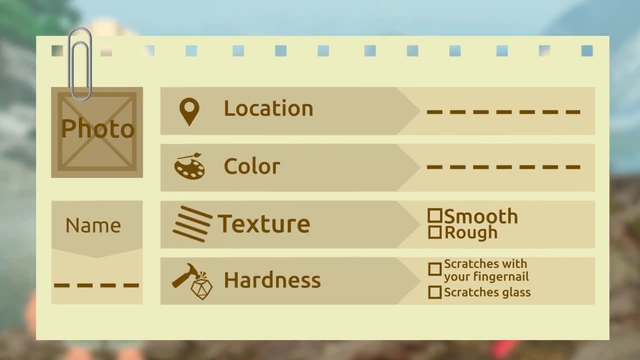 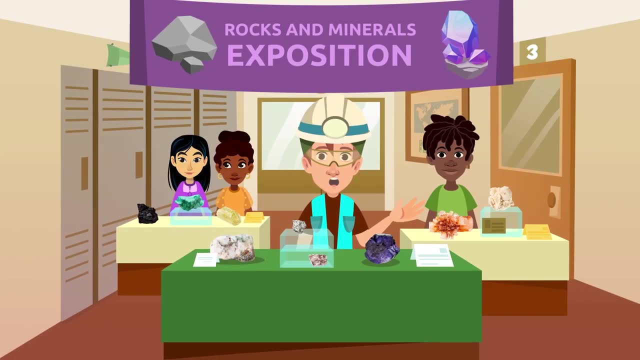 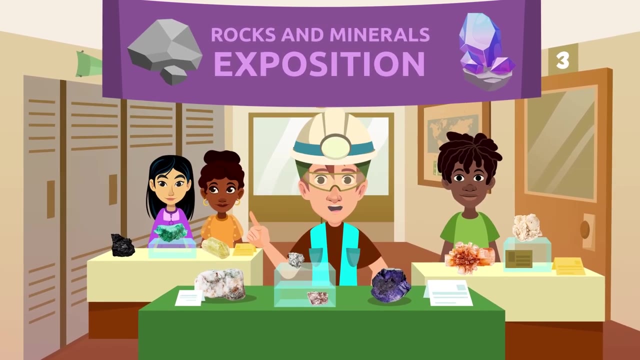 Color Texture: Smooth, Rough Hardness- Can scratch it with your fingernail. It scratches the glass. The exposition was a huge success. Today we learned that rocks are formed from minerals and that both rocks and minerals are part of nature. 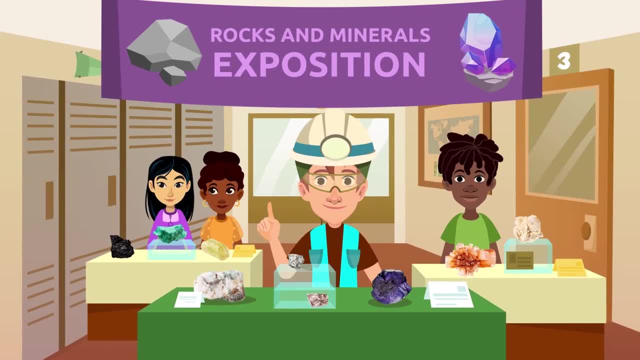 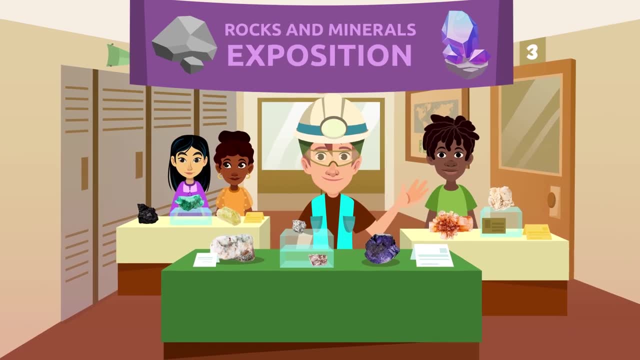 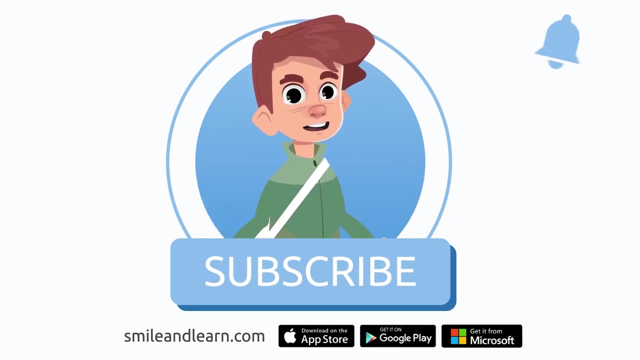 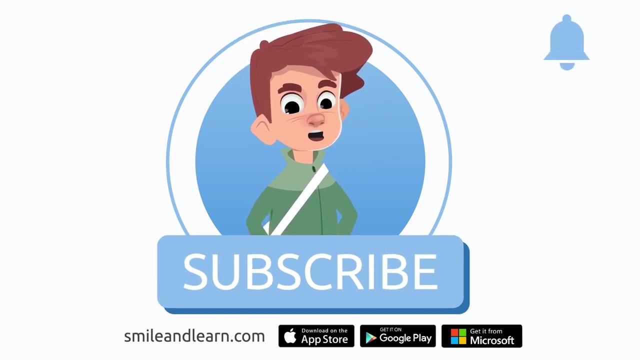 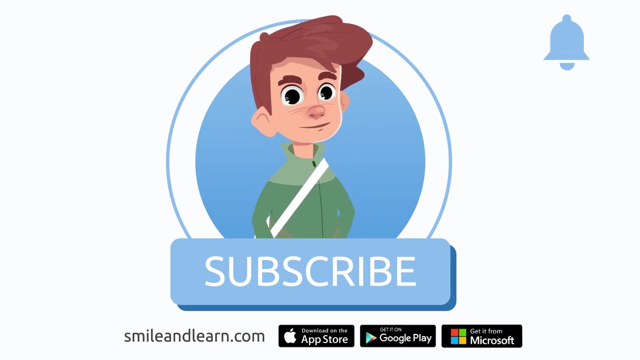 and the landscape that surrounds us. If you want to learn more about rocks and minerals, watch our upcoming videos. We've learned so much in just one video. Did you know there are many more videos? Imagine how much you could learn. Subscribe to the Smile and Learn educational channel to learn and have fun at the same time.